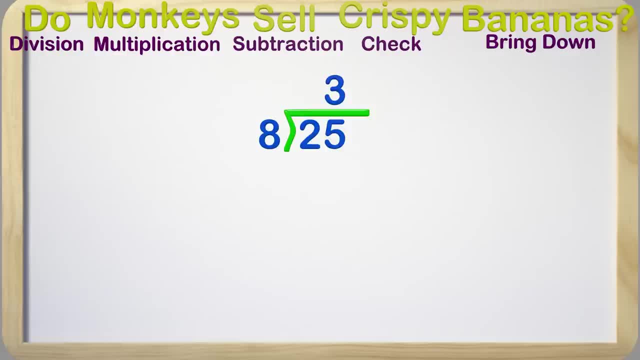 We divide it and now we do multiplication 3 times 8 is 24, and it goes directly under the dividend of 25.. We now move on to subtraction: 5 minus 4 equals 1, and 2 minus 2 is 0.. 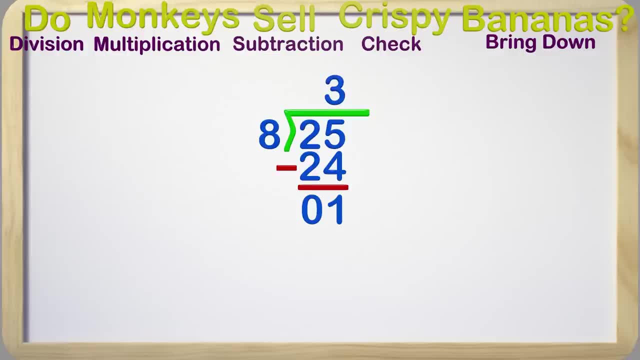 Our next step is to check and see if 8 goes into the number we just got, which is 1.. The answer is no: 8 does not go into 1 because 1 is smaller than 8.. The last step is to bring down. 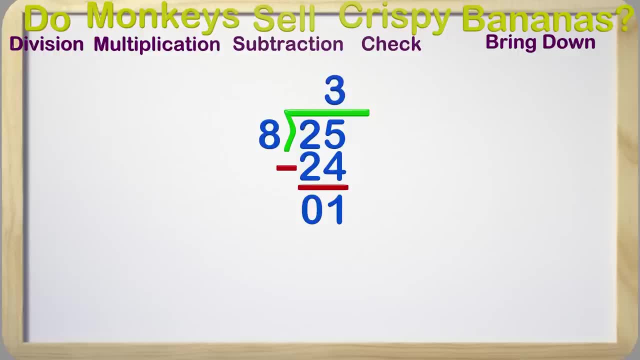 But there is nothing left to bring down. The question is: what do we do with our leftover or remainder? We will take this number 1 and put it up here with our answer. The letter R means remainder and the 1 is what was remaining after solving the problem. 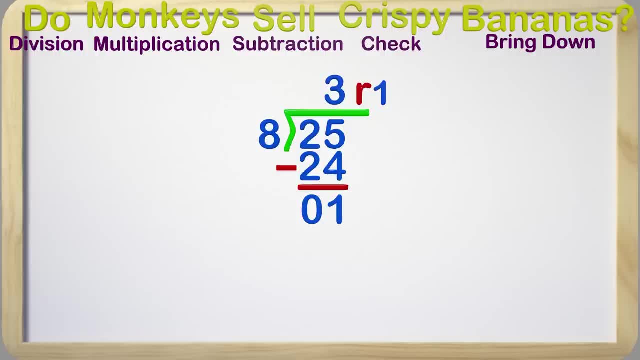 So the quotient or answer is 3 with a remainder of 1.. We now know that 8 goes into 25, three times with a remainder of 1.. Great job, guys. I am feeling so much better already. Let's do one last problem today. 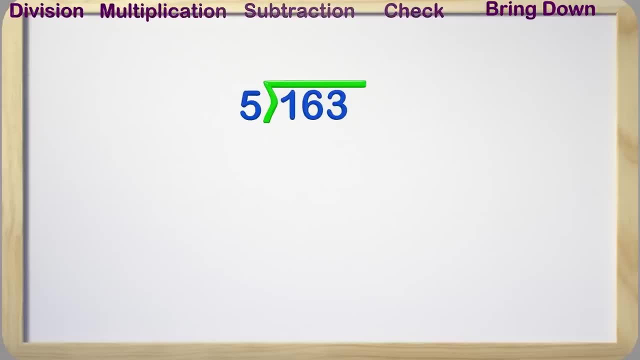 163 divided by 5.. Now this might look scary, but taking it step by step will make it easy. Pause the video and work the problem on your own and come back and join me. The first step is to ask if our divisor of 5 goes into the first digit, which is 1.. 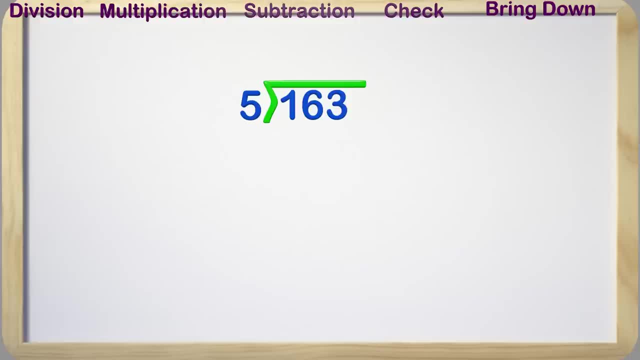 The answer is no, so we put a 0 up top or leave it blank and pull in the next digit. Does 5 go into 16, and if so, how many times? The answer is 3 times. Now we multiply. 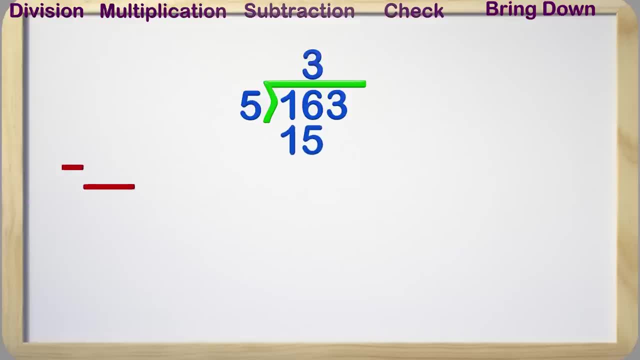 5 times 3 gives us 15.. Now we subtract 16 minus 15,, which gives us 1.. We check if 5 goes into 1, which it does not. so we are doing good, and the last step is bring down. 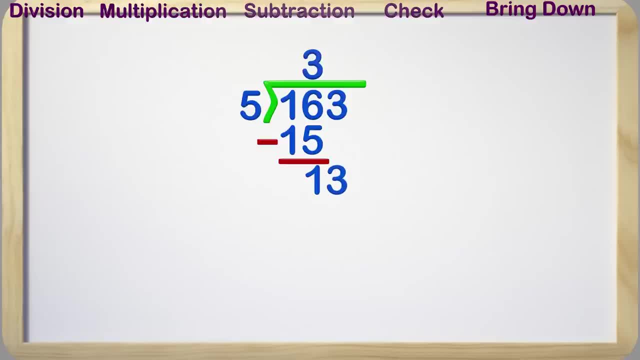 We bring down the 3, and it makes 13.. We start the steps all over again with division. How many times does 5 go into 13 without going over 2 times? so we write the 2 above Now. we multiply 5 times 2,, which gives us 10.. 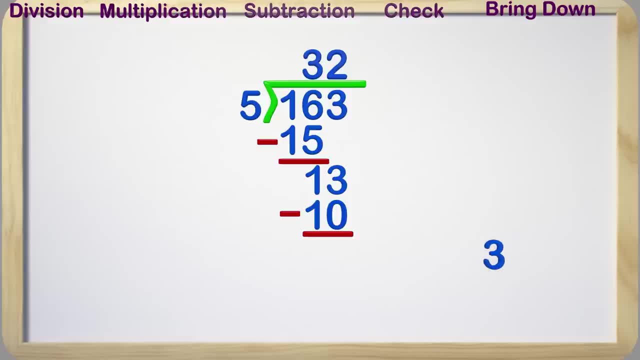 Subtraction is next, and 13 subtract 10 is 3.. The next step is to check: Does 5 go into 3, and the answer is no. The last step is to bring down. but there is nothing left to bring down, so we are done.